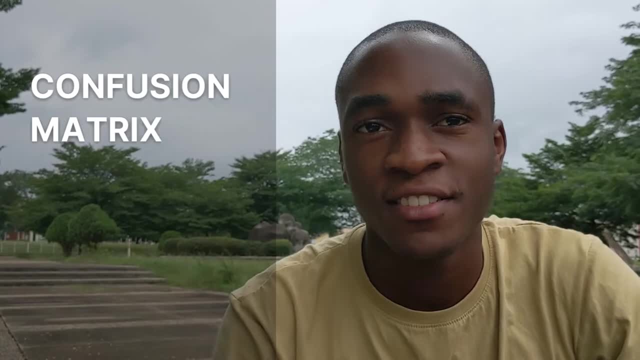 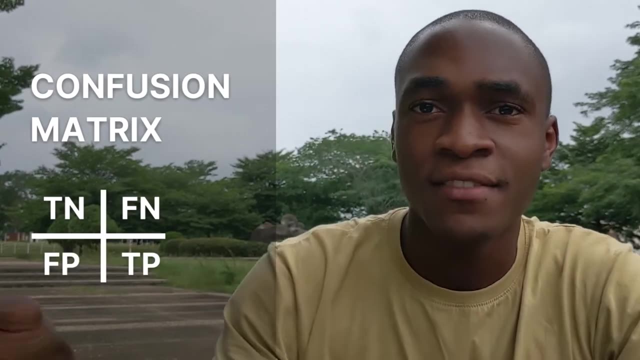 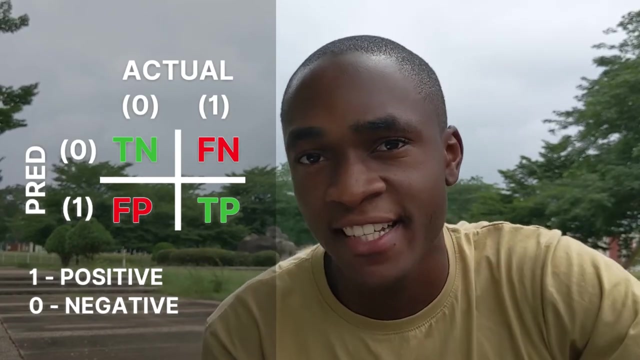 explain. this is what's called a confusion matrix. any confusion matrix is just simply a two by two dimensional matrix that shows your true negatives, false negatives, true positives and false positives. True negatives are examples that your algorithm thought were negative and we're actually negative, while true positives, on the other end, are examples that your algorithm thinks. 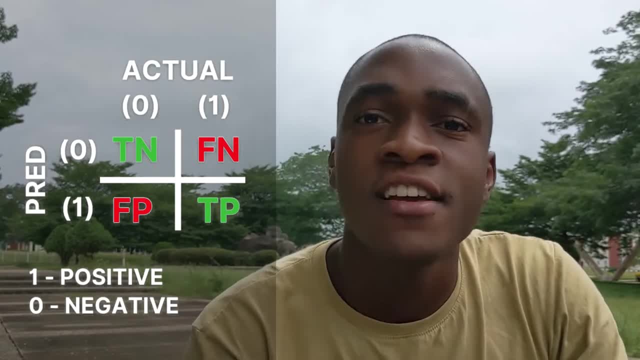 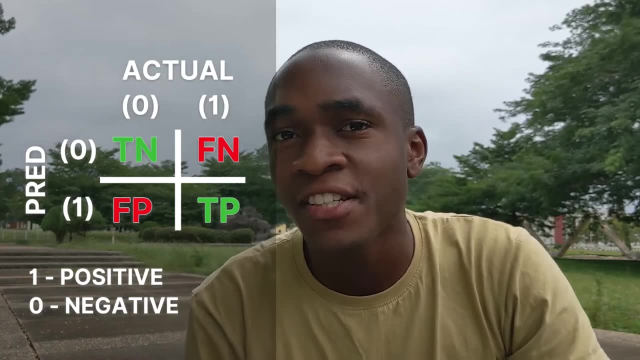 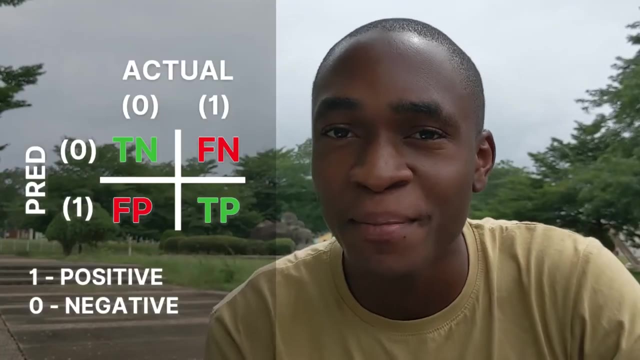 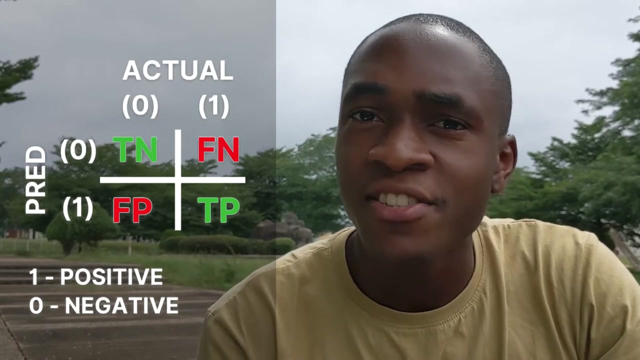 are positive and were actually positive, so you got it correctly. False negatives, on the other hand, are examples that your algorithm thought were negative, but they were actually positive, so you got it wrongly. I mean, it missed it. More concretely, false positives are those that your algorithm thinks are positive, but they were actually 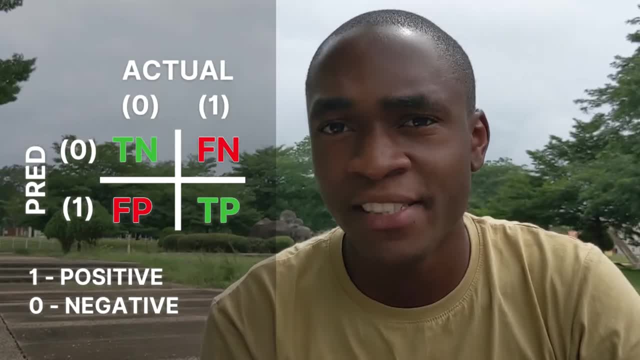 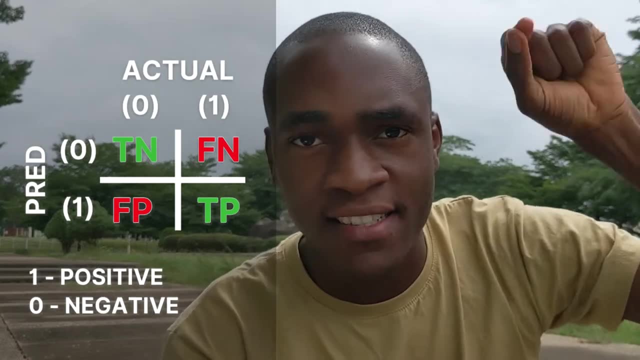 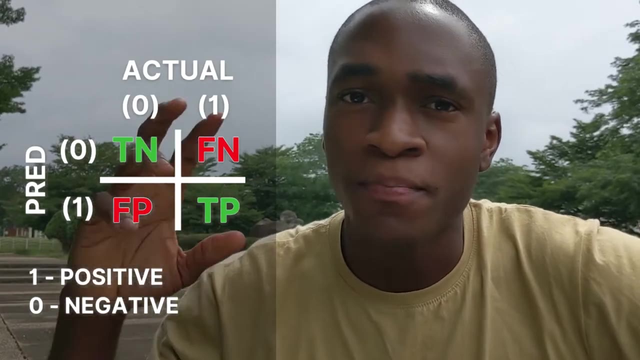 negative, right? yeah, so when i draw my confusion matrix, i actually have my actual labels on the x-axis like this and predicted on the y-axis. so i mean, that's, that's what works for me. you could, you could do it the other way. i've seen, i've seen um other blogs, other tutorials, did the other way. 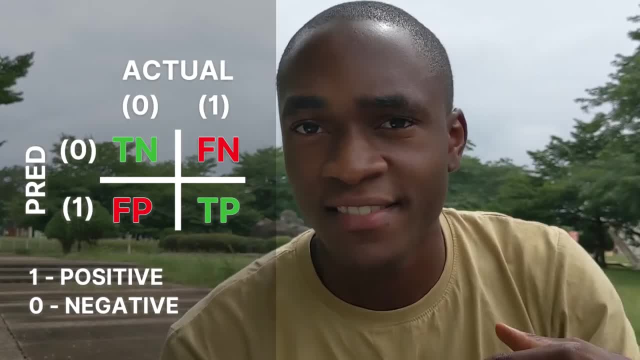 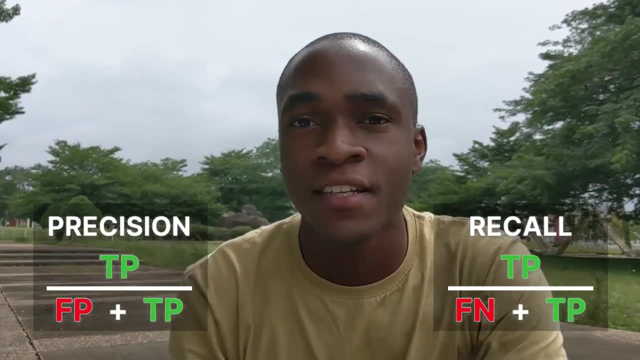 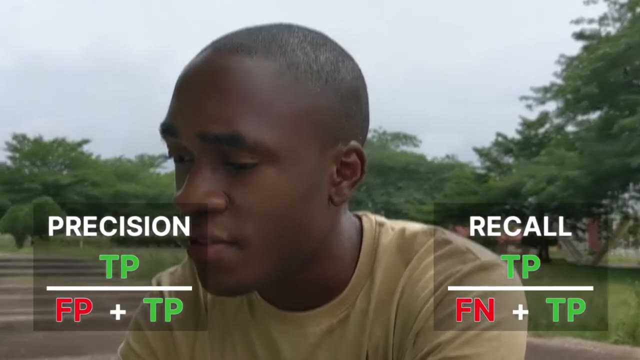 like i've predicted, at the top and actual on the sides. but this is what works. back to position. you know, position is true positives divided by false positives plus true positives, while recall is false positives divided by true positives plus false. wait what the? so recall is true positives. 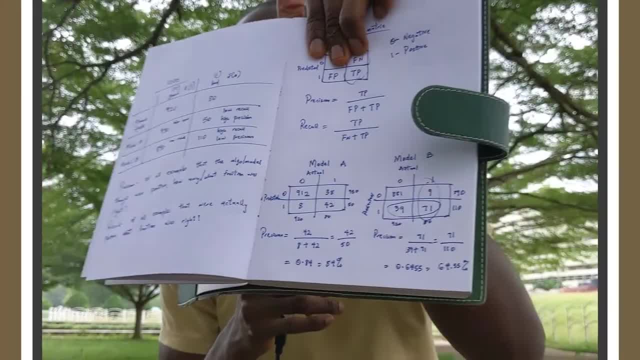 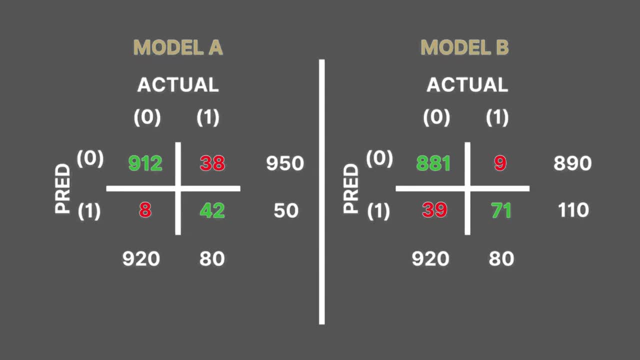 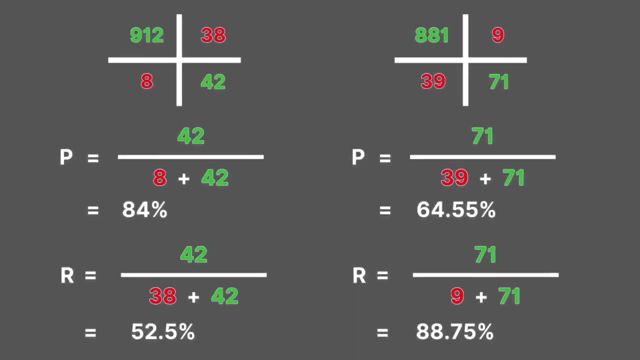 divided by false negatives plus true positives. real quick, let's run some numbers. these figures are hypothetical but they pretty much represent, you'd see, in a normal confusion matrix, and when you calculate the precision and recall from the formulas that i gave earlier, you discover that model a has higher precision, lower recall and 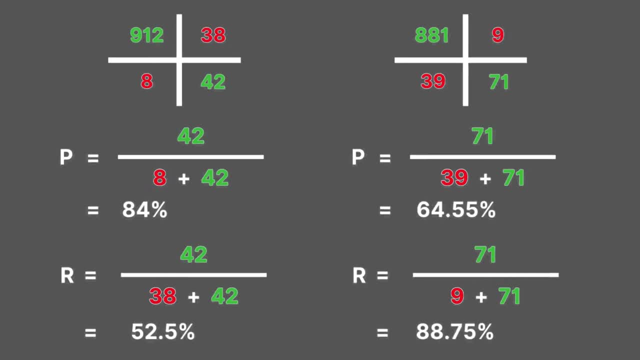 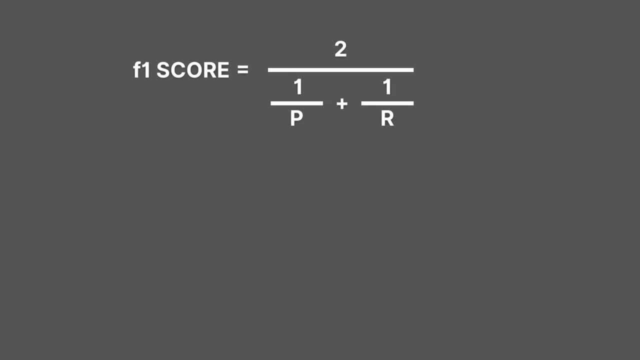 model b, which is on the right side, has a lower precision and an higher recall, and then this leads to what's called an f1 score, and f1 score is pretty much just- uh, it's more like an average of your precision and recall. model b is kind of like better than model a.